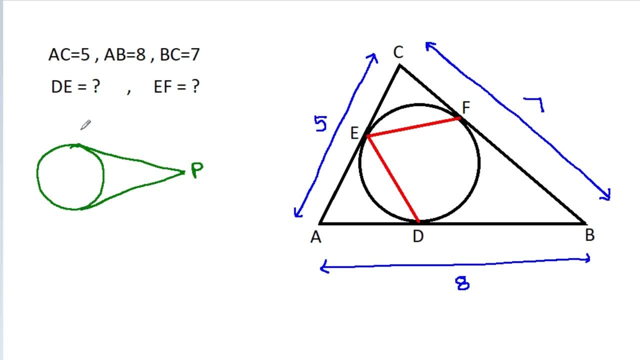 on the circle. suppose this point is A and this point is B, Then P is equal to 0. If B is equal to BA, it will be equal to PB. So here, from point A, if AD is A, then AE it will be A. 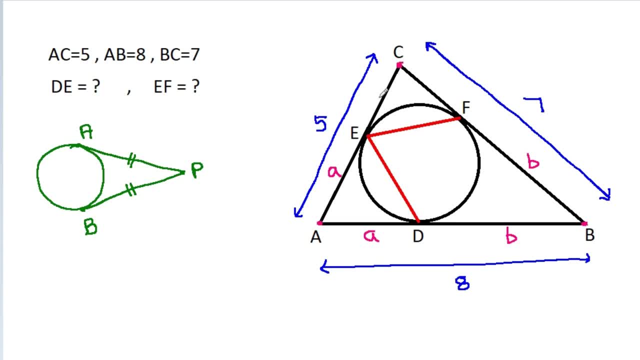 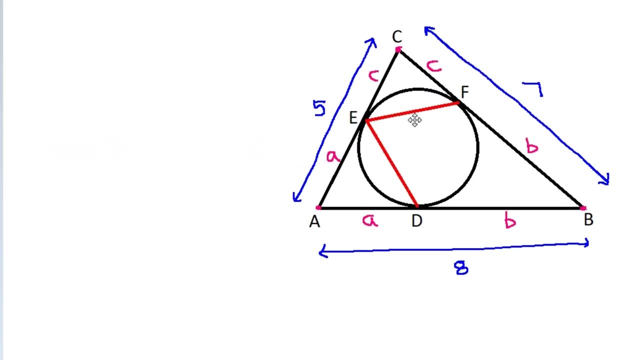 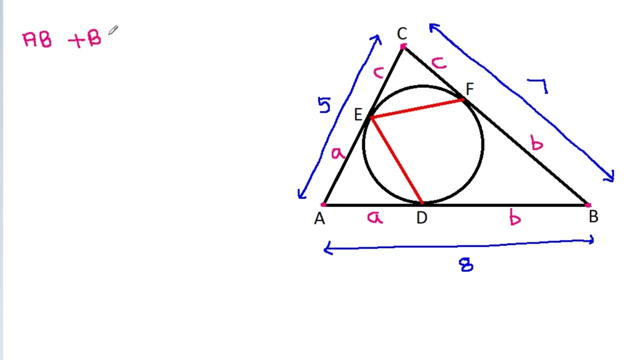 and from point B: if BD is B, then BF it will be B, and from point C, if CE is C, it will be R, or P, then CF it will be also C. And now AB plus BC plus CA, it is equal to 8 plus 7. 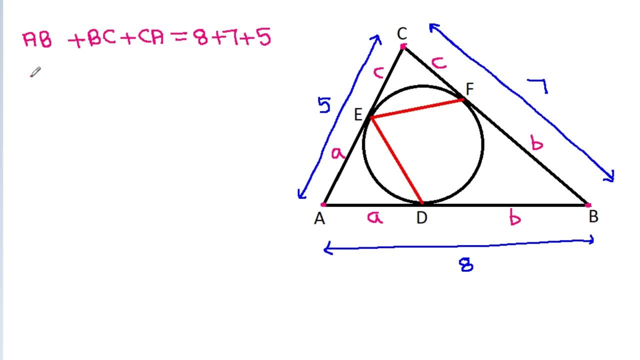 plus 5. And AB it is A plus B plus BC. it is B plus C plus CA, it is C plus A. that is equal to 20.. And it is 2A plus 2B plus 2C is equal to 20.. So A plus B plus C it will. 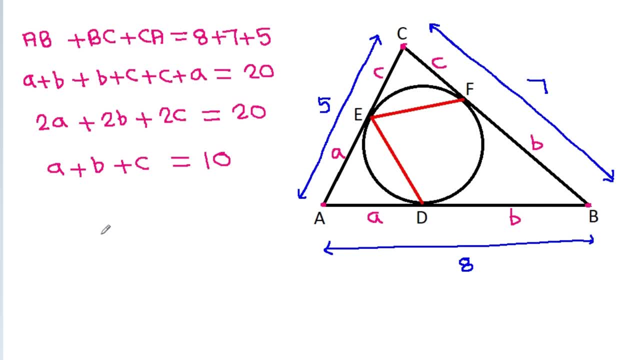 be equal to 20.. 10 and we have A plus B is equal to AB, that is 8, B plus C is BC, that is 7, and A plus C it is AC, that is 5, and we have A plus B plus C is 10. so from these two equations we can: 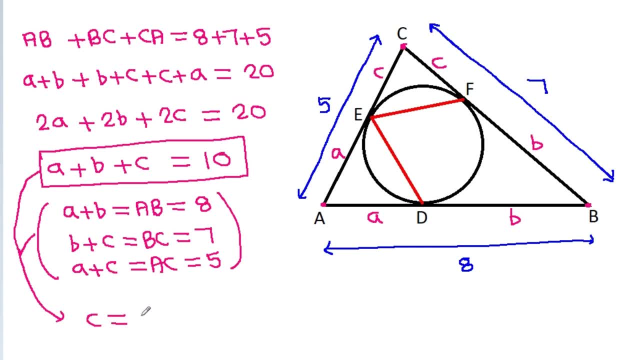 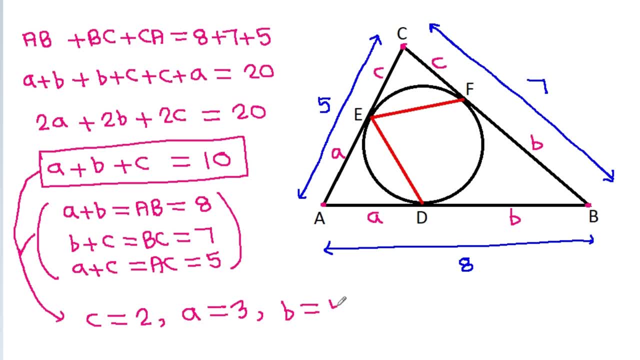 10 minus 7, that will be 3, and B is equal to 10 minus 7, that will be 3, and B is equal to 10 minus 5, that will be 5. so we get: A is 3, B is 5 and C is 2, and. 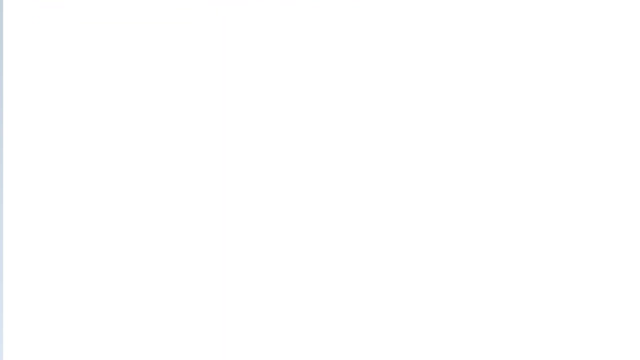 B is equal to 10 minus 7, that is 11.. Now in an iterangle: A, B, C: if AB is A, AC is B and BC is C and D is A. Now in an iterangle: A- B, C: if AB is A, AC is B and BC is C and D is A. 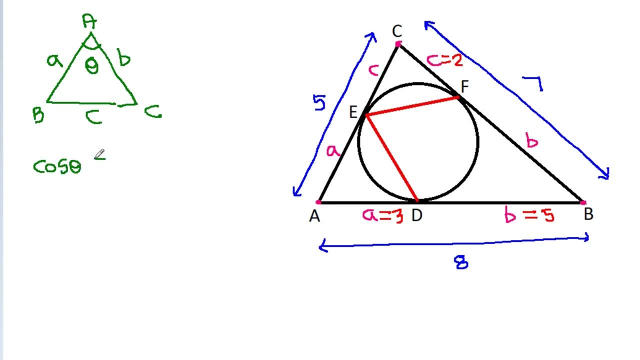 and BC is C and D is A. angle is theta, then cos theta, it is equal to a squared plus b squared minus c squared by 2 ab. so here, suppose this angle is alpha, then cos alpha it will be equal to ab squared plus ac squared minus bc, squared by 2 times ab squared minus c square. 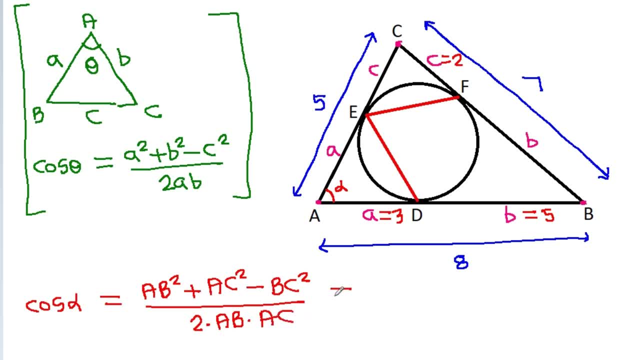 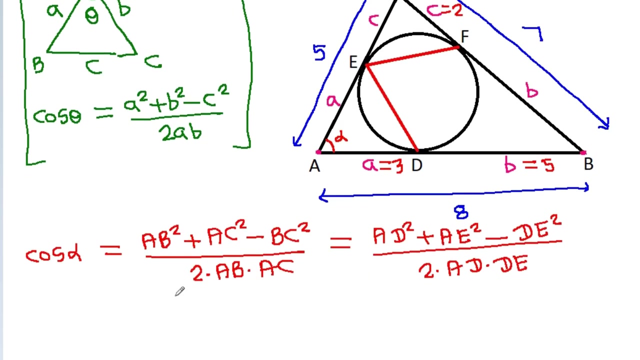 times AC and it will be also equal to AD square plus AE square minus DE square by 2 times AD times DE and AB, it is 8A. square plus AC is 5A. square minus BC is 7A. square by 2 times AB is 8 times AC is 5.. 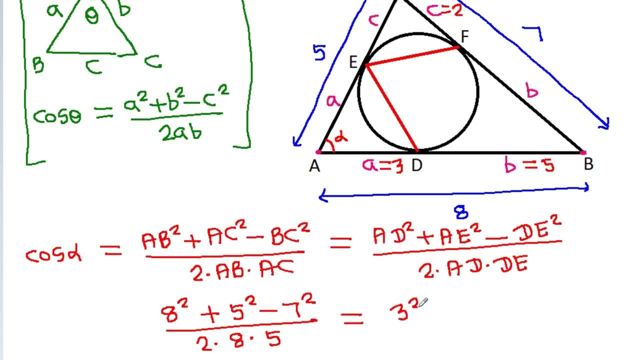 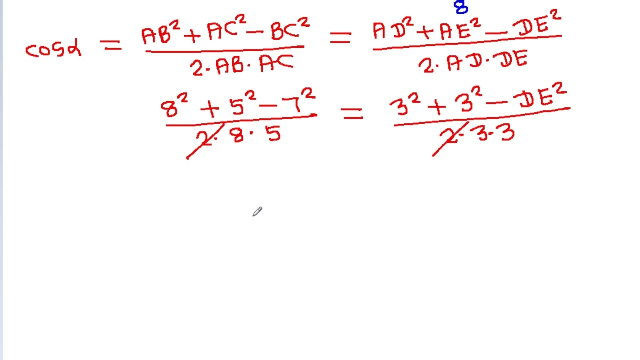 It is equal to AD times DE. AD is 3A square plus AE. it will be also 3A square minus DE square by 2 times, 3 times 3, and 2 will get cancelled and it is 64 plus 25 minus 49.. 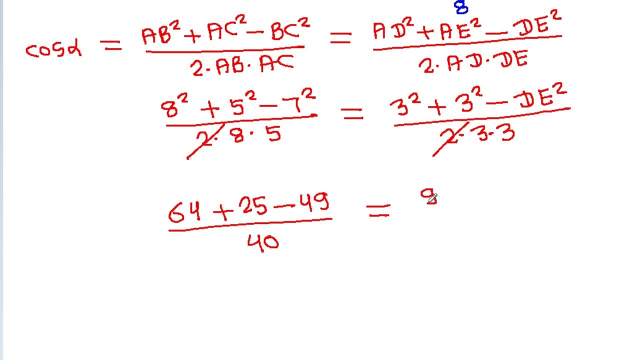 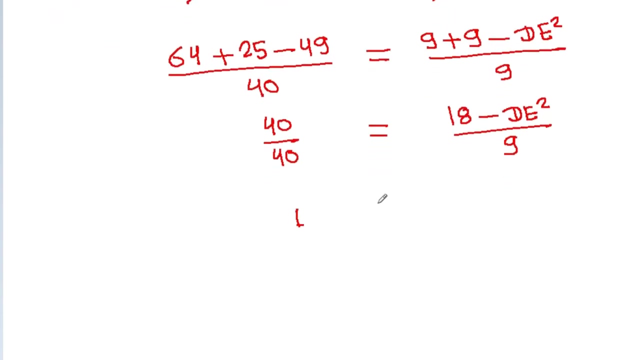 40 is equal to 9 plus 9 minus DE square by 9 and 64 plus 25 minus 49.. It will be 40 by 40.. It is equal to 18 minus DE square by 9.. And it is 1 is equal to 18 minus dE squared by 9.. 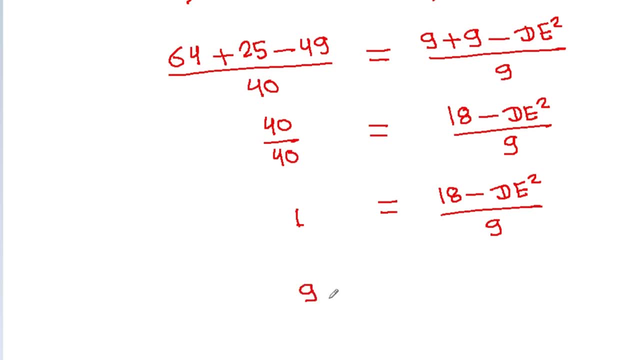 And if we cross multiply, then 9, it will be equal to 18 minus dE squared. So dE squared it will be equal to 18 minus 9.. And dE squared it is equal to 9.. 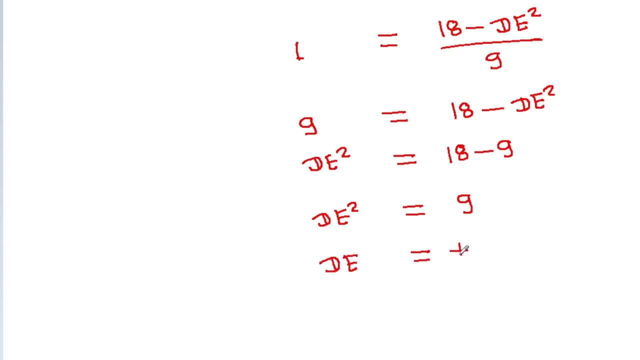 So dE it will be equal to plus minus s square root of 9.. That will be equal to plus minus 3.. And dE it is equal to 18 minus 9.. So dE squared, it is equal to 18 minus 9.. 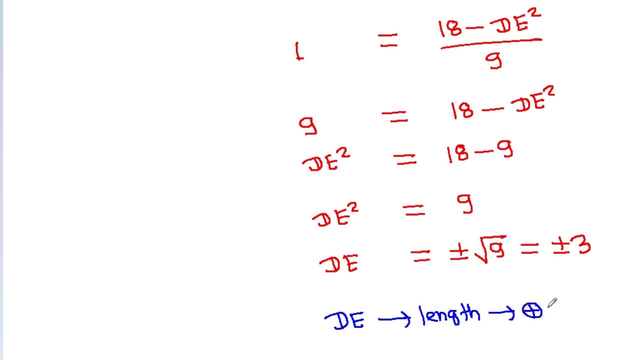 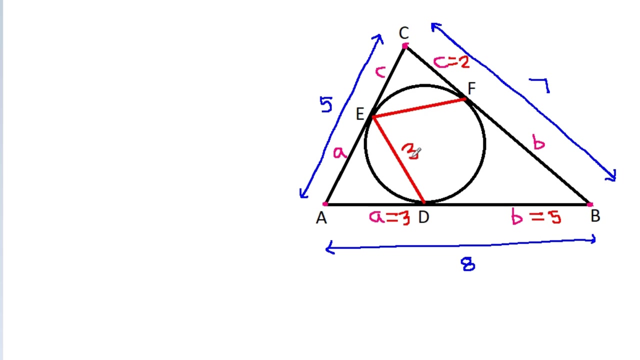 Length. that should be positive, Hence dE. it will be equal to 3. And we have, dE is 3.. And now suppose this angle is beta, Then cos beta, it will be equal to AC squared plus BC squared minus AB squared by 2 times AC times BC. 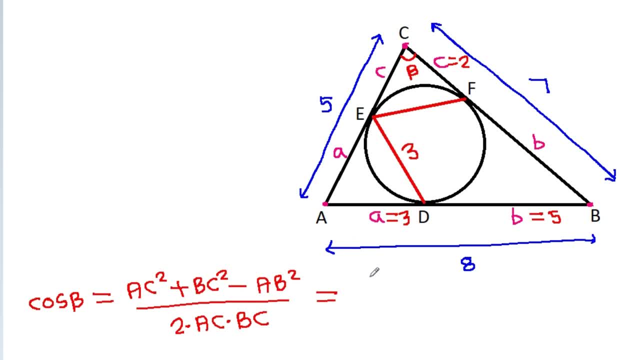 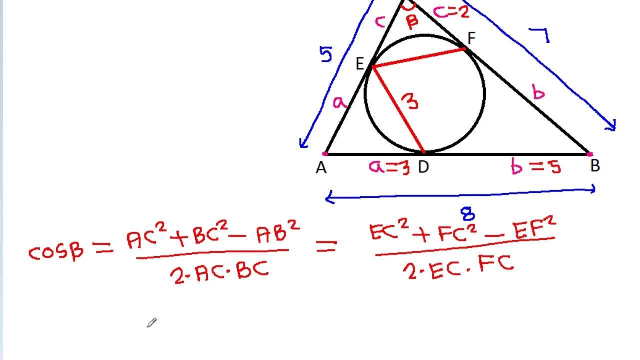 And it will be also equal to EC squared plus FC squared. And it will be also equal to AC squared minus EF squared by 2 times EF squared by 2 times EC times FC And AC is 5A squared plus BC is 7A squared minus AB is 8A. squared by 2 times AC is 5A squared. 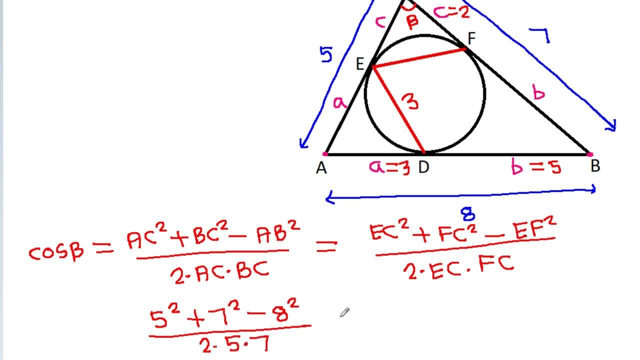 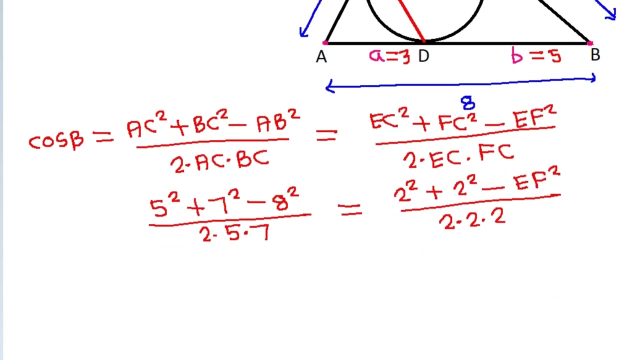 And AC is 5 times BC is 7.. It is equal to EC. it is C. that is 2A squared plus FC is 2A squared minus EF, squared by 2 times 2 times 2.. And 2 will get cancelled. 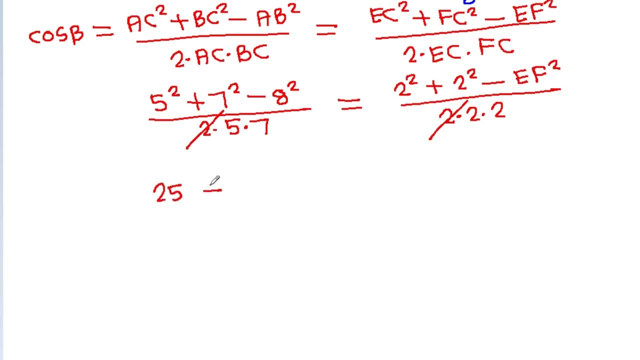 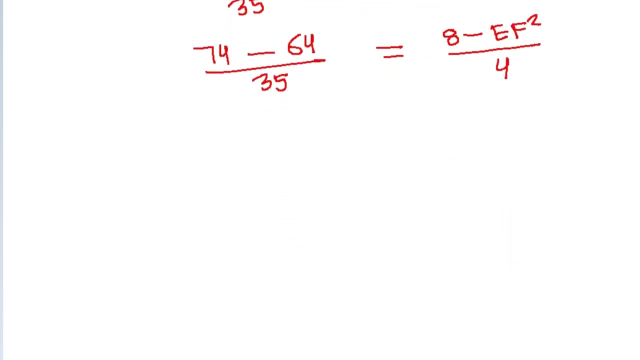 and it is 25 plus 49 minus 64 by 35 is equal to 4 plus 4 minus EF square by 4, and 25 plus 49, it is 74 minus 64 by 35, it is equal to 8 minus EF square by 4, and it is 10 by 35 is equal to. 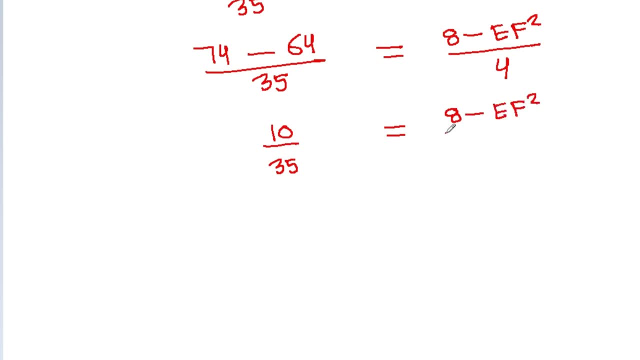 8 minus EF square by 4, so 10 by 35 times 4, it will be equal to 8 minus EF square, and 5 times 2 is 10. 5 times 7 is 35, so it is 8 by 7 is equal to. 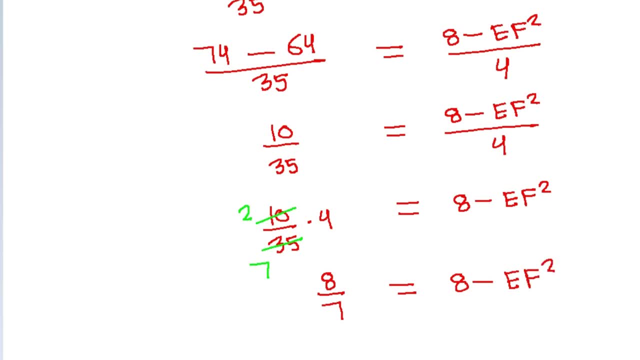 8 minus EF square. so EF square it will be equal to 8 minus 8 by 7 is equal to 8 minus EF square. so EF square it will be equal to 8 times 1 minus 1 by 7 and EF square it is 8 times 6.